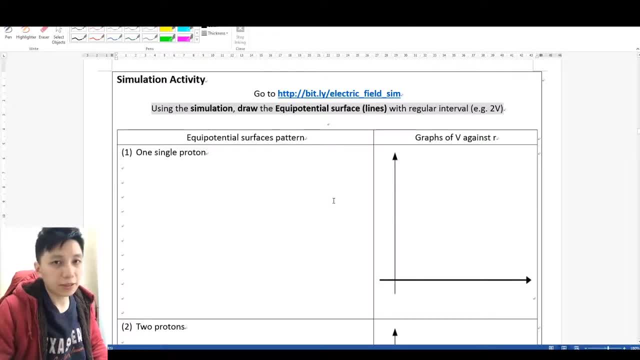 Hi, let's have a simple and interesting simulation activity. We'll be using the simulation from PHET- I've put the link here on the worksheet already- And we'll learn about something called the equal potential surfaces or equal potential lines, which is a line joining the same potential simply, And also see how that can help you to convert into the graph of electric potential against distance. So I'll show the first one. There are three examples in 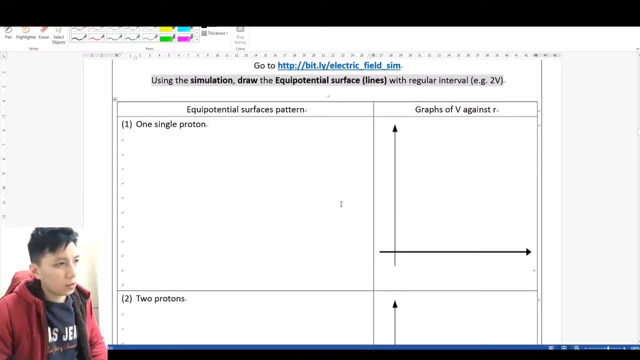 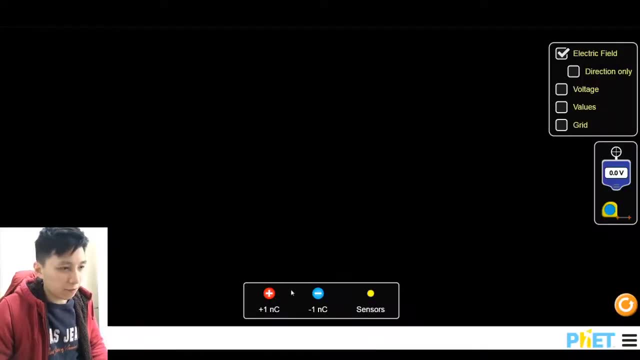 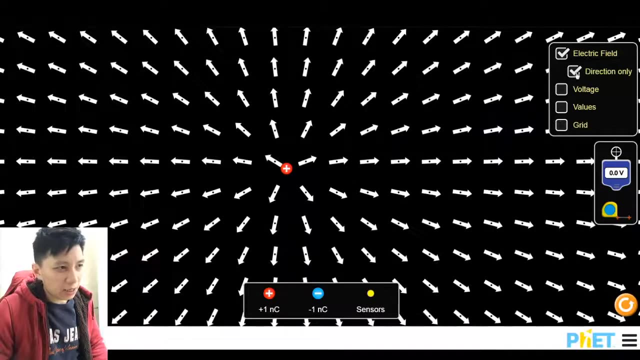 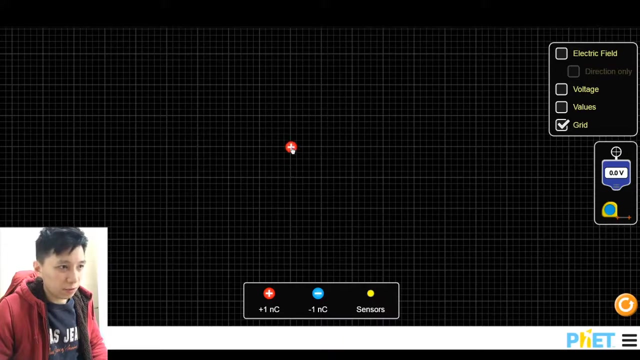 total. I'll show you the first one as an example. So the first case is having only one single proton or positive charge. So here in the simulation environment, you can drag this positive charge out. Okay, and this is what you see. I will recommend you to enable. Actually, you just need to agree. I think right, you don't even need the electric field line. All right, or if you like to, then yeah, it's up to you. I will probably try to put this. 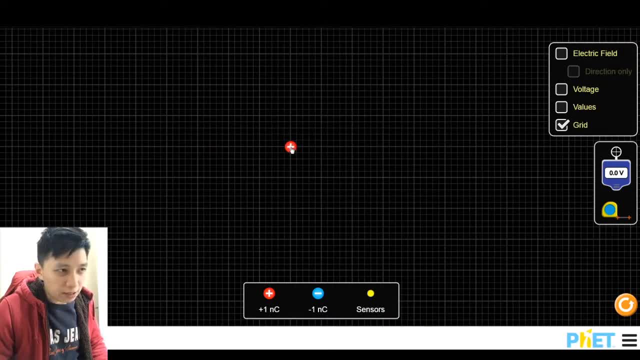 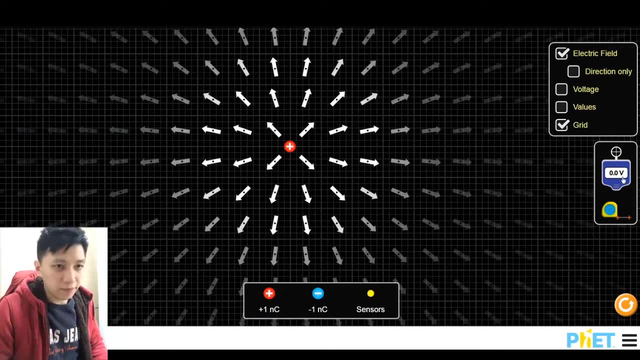 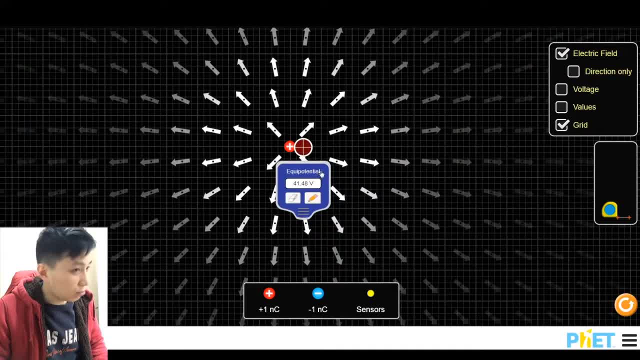 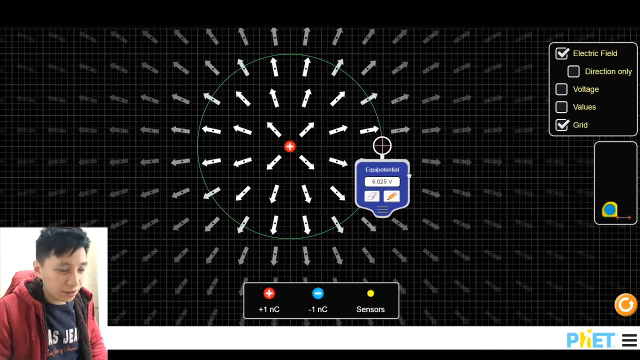 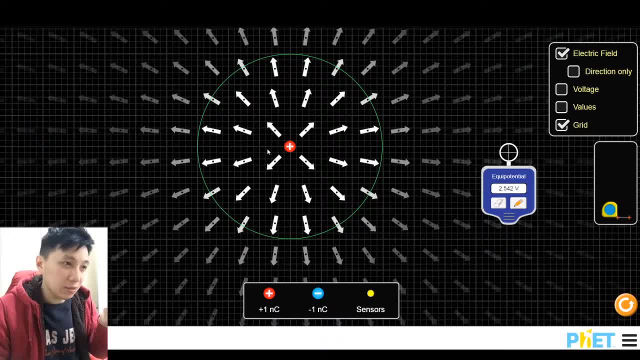 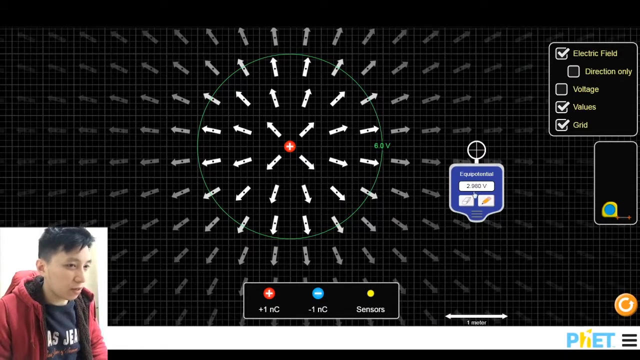 can see that the potential is not exactly the same. So you can see that the potential is not exactly the same. So you? so what I want you to do next is go and set a regular interval. so in the worksheet I suggest you maybe set 2v. so it's up to you. you can set 2, you can set. 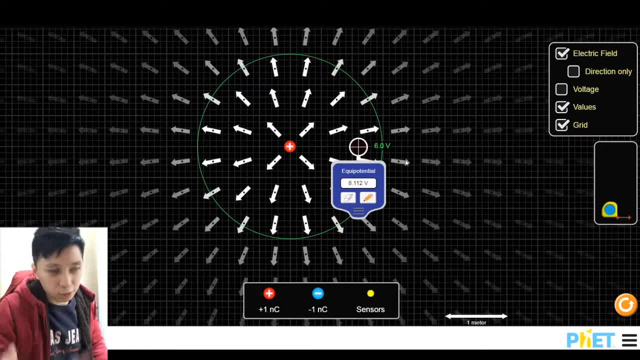 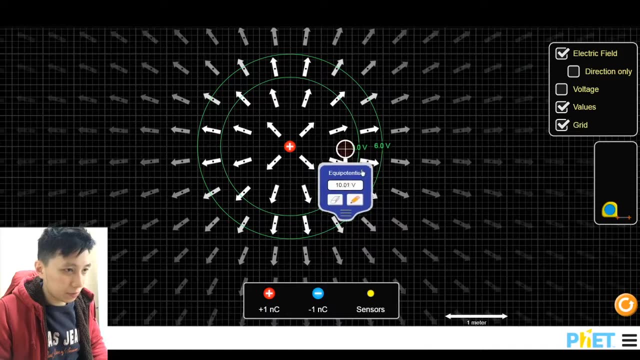 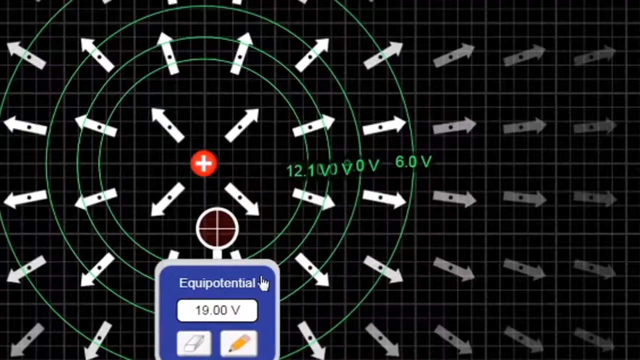 3. you can set 1 if you would like to spend more time. I think 2 is pretty good enough, so let's do this. yeah, so this is close to 8.0, okay, so again you see another circle and let's do more. next is 12. ah, 12.1, nevermind, okay, so if you see, 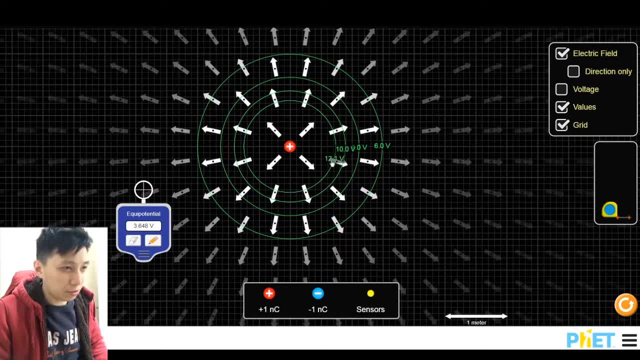 the words are overlapping is not easy to read. what you can actually do is you can drag them. okay, it's pretty cool. this simulation is pretty well designed. so sorry for 12.1. I think you understand right. 12.0 is somewhat a bit outside right from. 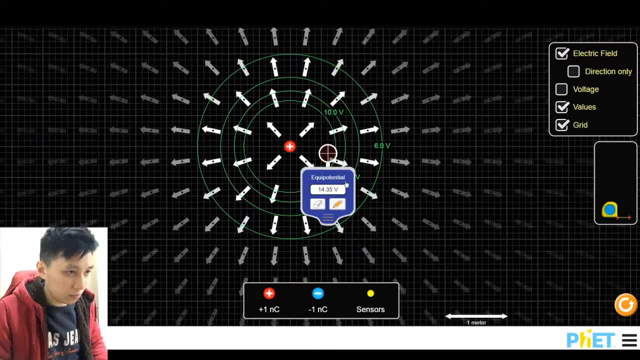 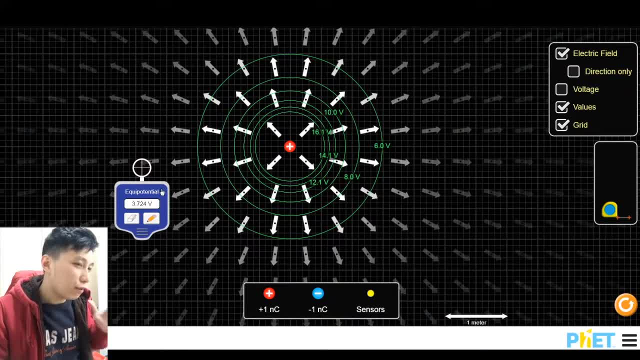 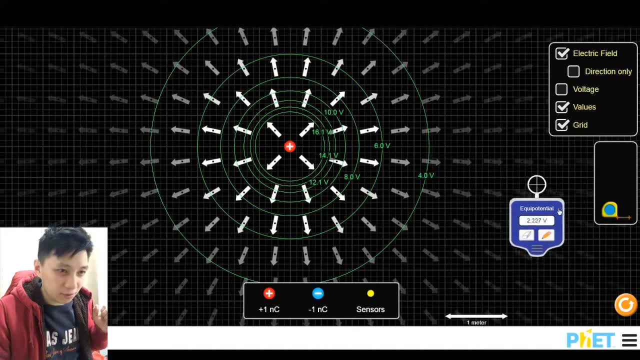 okay, nevermind 16.1. okay, nevermind 16.1, 16.1, 16.1, 16.1, 16.1. so after you have done this or if you like to, you can do more like four. okay, outside is easier. four and then two. hopefully I can still show it. yeah, I can. 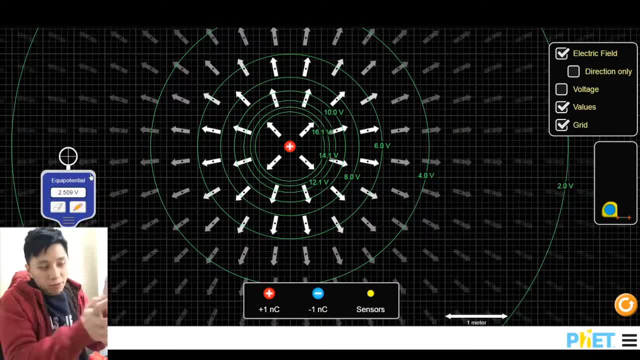 Wow, exactly two. so you can see this is a pattern. Wow, very cyber, but, by the way, cyberpunk. and so you can see the most interesting pattern is it get shorter and shorter for each circle when you get close to it, and that's something related to, again, how the V will change against the out. so this is a pattern. 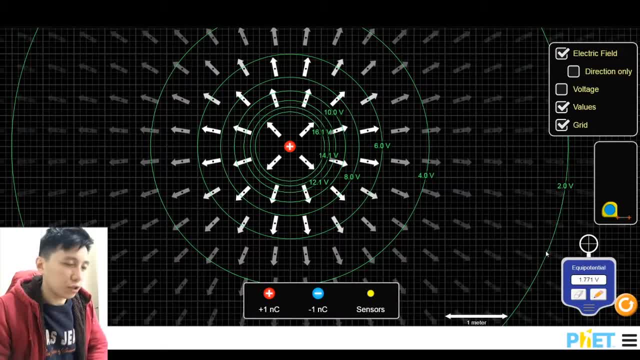 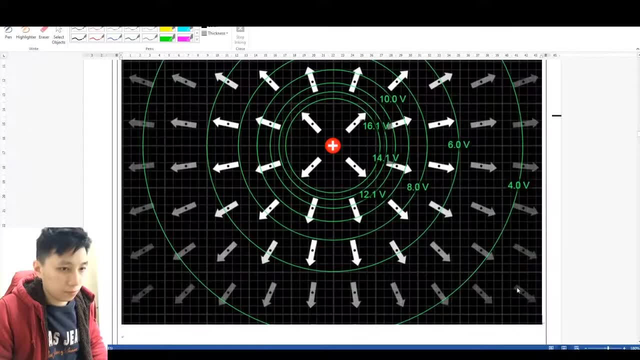 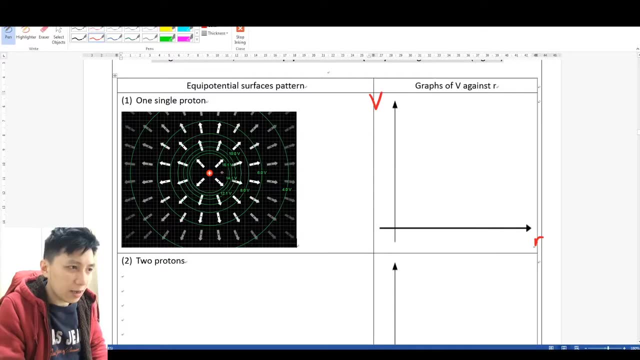 that I would like you to draw on your worksheet, or if you're doing it on the computer, then just screenshot it. easy-peasy, all right. moving to a graph, let's put down the axis first and let's say, if I call a positive charge or the other proton is at the middle, okay, so this is where it. 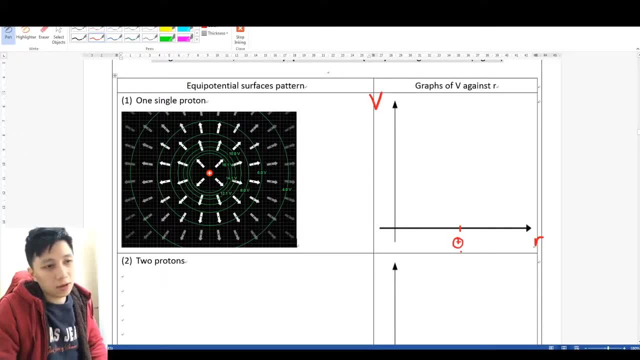 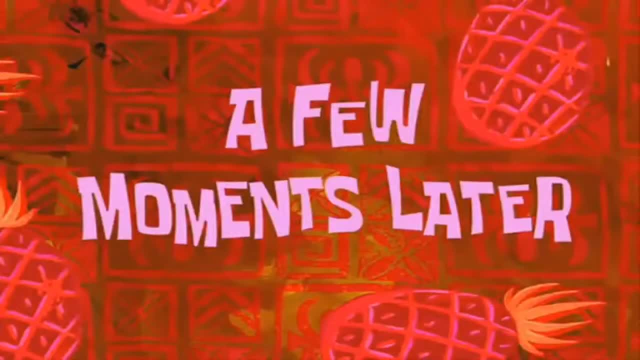 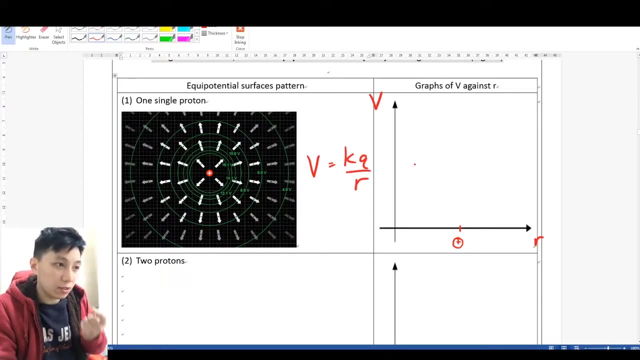 is located at then how are you going to draw the graph of this? pause the video and try it yourself a few moments later. once again, we can recall the equation that is: V equal to K, Q over R. R is the distance between the point charge and the external charge, like the proton here, and so when you get close to 0 and get, 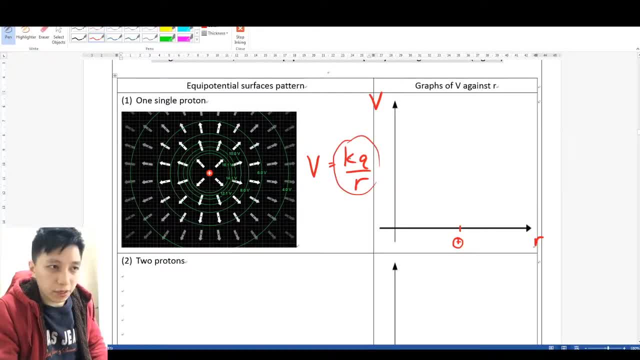 close to the proton, the whole thing will become infinite, or getting close to infinite, and therefore what you will have to do is you should draw an absinthe- something you learn in math, I believe, and that should be something you should get close with. okay, so probably something like this: symmetrically, and it: 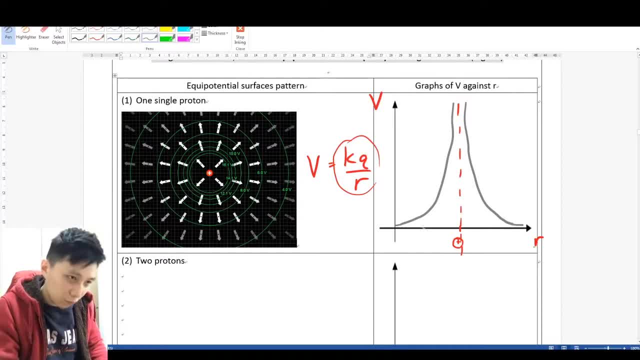 should tends to be like to zero, right it, your verge, converge to zero on to side. and, of course, in your mind you should relate the idea of: like this voltage, it changed much faster than the outer one by looking at this and this, okay. when you look at the change in Y, when it's closer, it changed much faster than the. 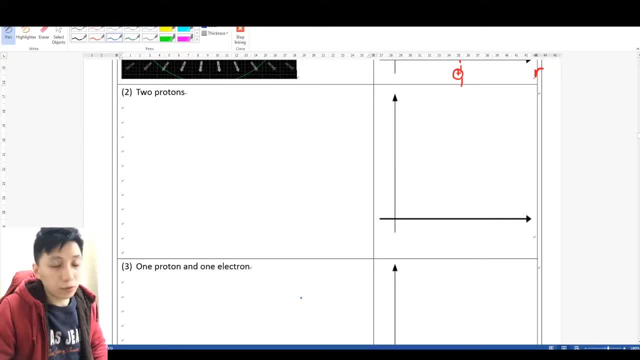 one, that is outside case number two: two protons. so never mind, this is wrong. this is the truth here. what you should do is you should look at this proton. then what you should do is you should find out, like right now. now go and do it yourself on the simulation. pause the video now. 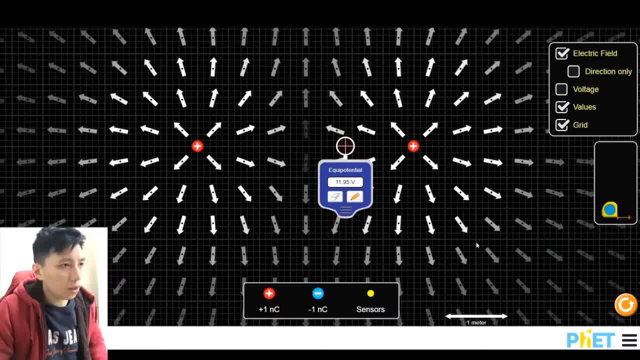 two thousand years later. let me also demonstrate. so here is how i place the two protons, and your decision may be slightly different and that would yield a different result in terms of the v and also the pattern size, like okay, but overall the whole pattern should be very similar. 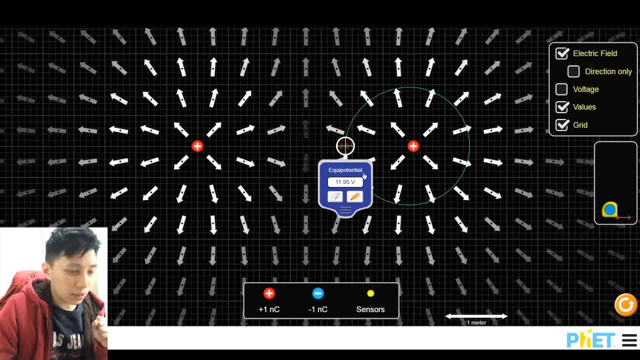 so, first of all, i've already located 12- okay, and i'm going to do it, and then you can see this is only locally here, and so i think there should be another 12. okay, right here, nice, and so i can go for 14 for each of them. so obviously the pattern is not going to be. 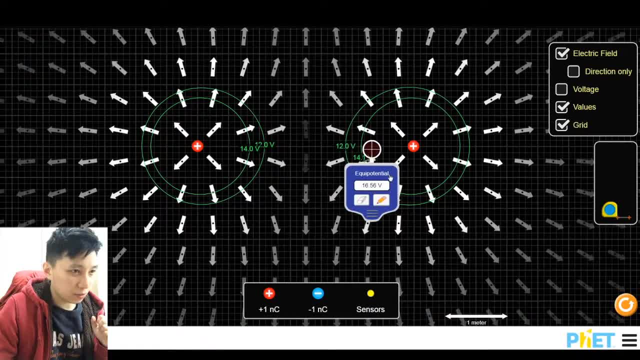 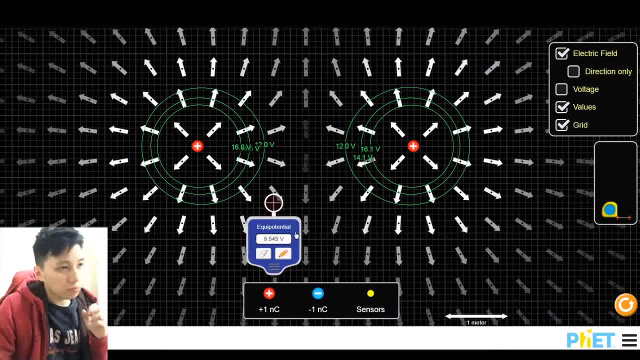 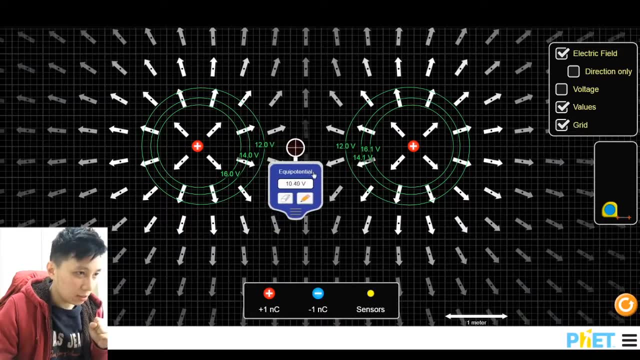 very surprising because that is similar to what you have in the first practice. okay, the most important pattern that you need to see is between them. so what happened in the space between them? and, unfortunately, if you try to search, like in, if you are following exactly my configuration or in your configuration, you'll find out. 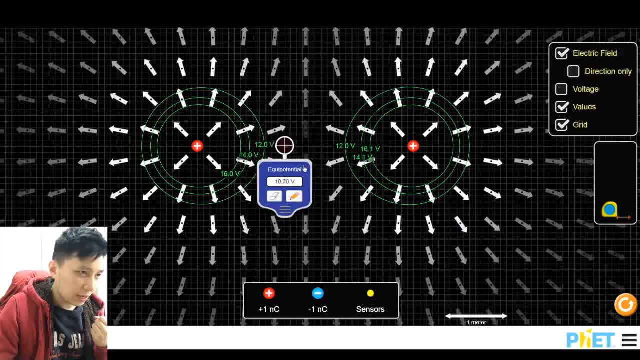 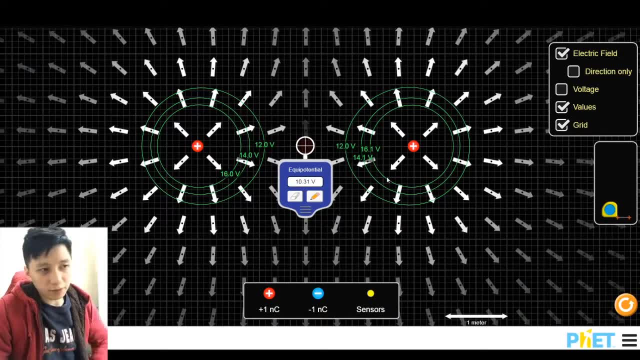 hey, if i want to locate 10, i cannot find it because the minimum between them is like 10.31 v. that is the minimum i can find. if i get closer to each side then it becomes higher again. so this is like the local minimum that you can have, and 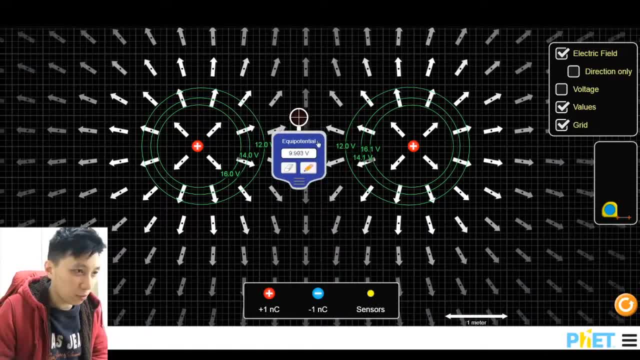 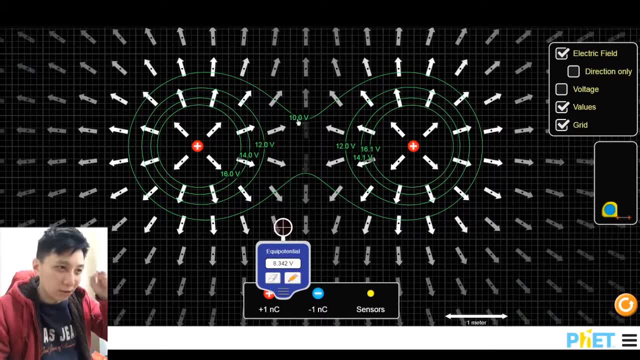 that's. that is what it is. so probably, what you have to do is go a bit higher and you'll be able to locate that, and so, in fact, the equal potential line for 10 v is somewhat like this, itself in the middle. so in the middle it's. 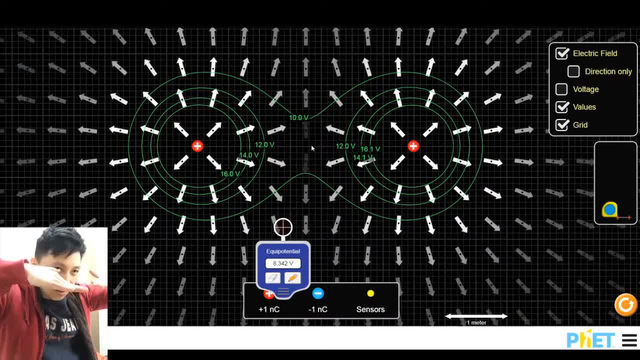 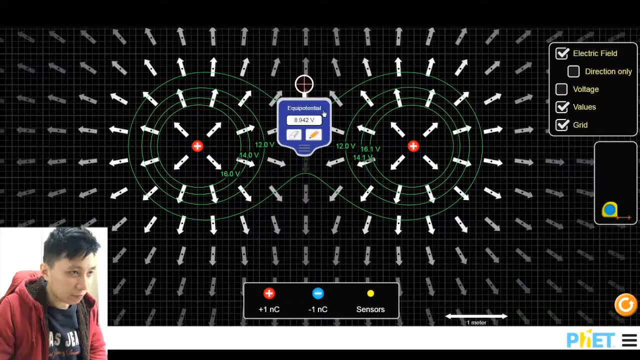 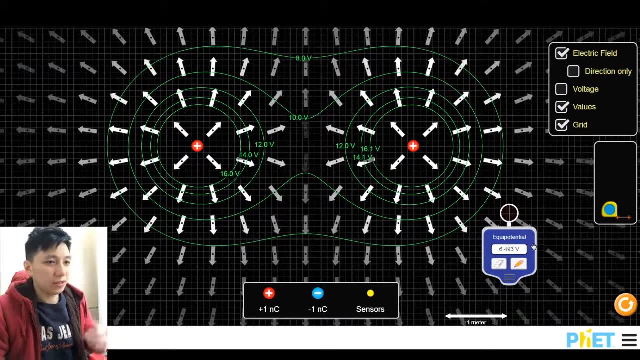 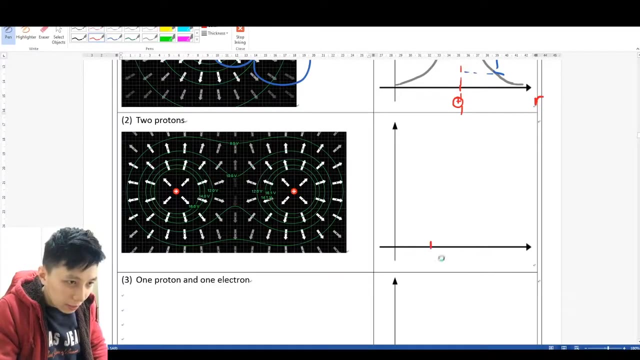 somewhat like it's still going down, but then it's not as low as 10.. all right, and so if i want to locate x, i guess i have to go for here. okay, something like this. so that is the pattern that you can find all right. so again, if i say here and here are the two positive charge, then how are you going? 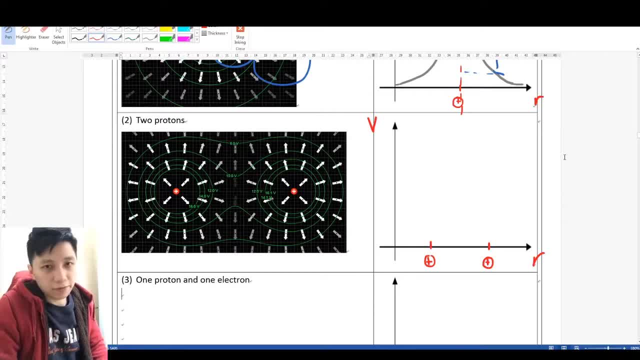 to draw the graph of v against out and pause the video now and try it yourself later. so, first of all, we can borrow from the idea that we just mentioned in the first case. so we'll have two asymptomes on each position and again: uh, they should look like this from infinity. 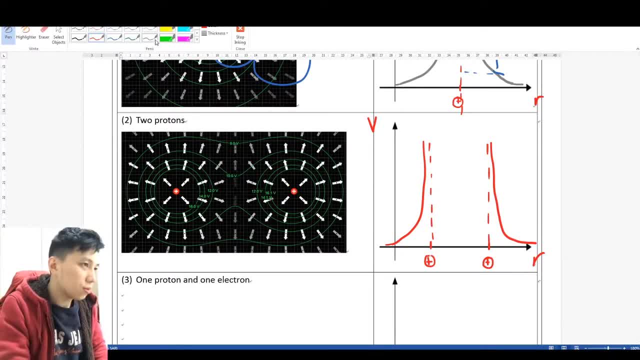 converge to zero and the most tricky thing is in between them. so, from what you have seen earlier, you would, you should see that it will go down up to a certain point and it will go back up again. okay, something like this: and if you really want to, you can indicate this value. uh, in our case it's. 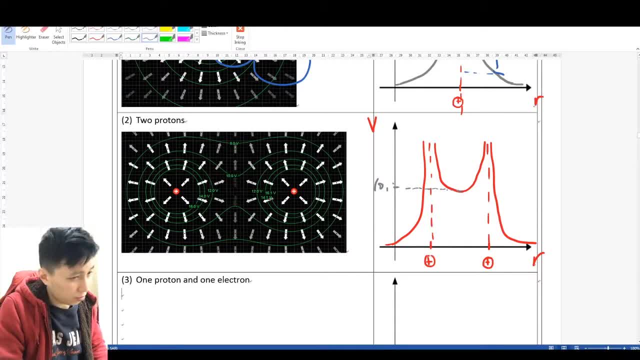 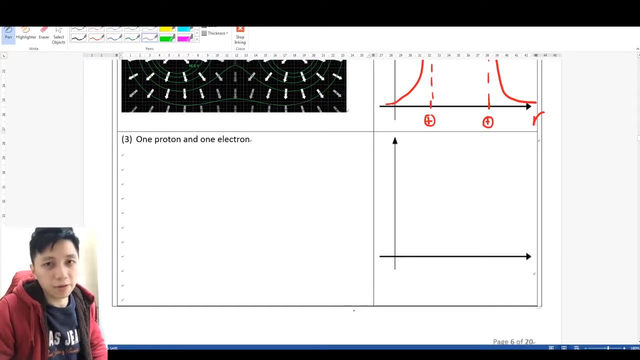 like 10 point, something right, 10.3 i remember. so yeah, just just a evaluate, depending on the distance between them, and yeah, that will be the local minimum of the potential between the two charges, okay, lastly, one proton and one electron. try out yourself on the simulation. pause the video now. 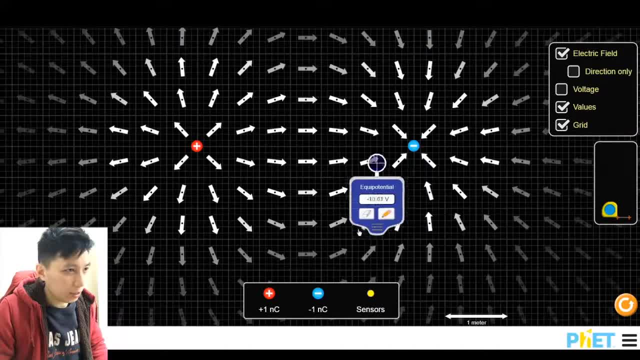 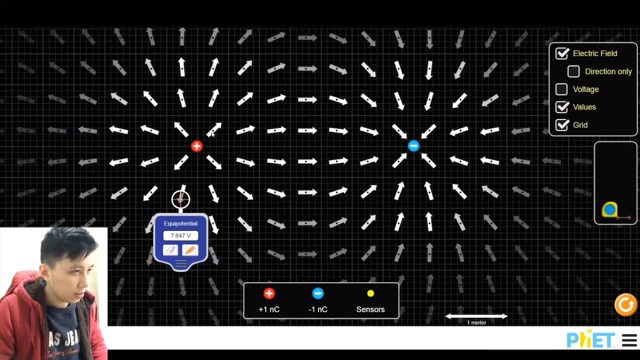 a few moments later. okay, let me try also. so here, by the way, you can also see the e-field, all right, if you have enabled it. all right, the e-field pattern, a bit similar to the magnetic field line, anyway. so here we have. the most interesting part must be zero, all right, if you remember what i said. 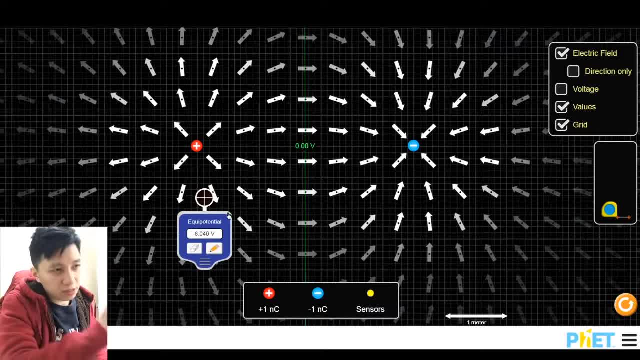 earlier in the previous video, when only 0 must be 0. if you remember what i said earlier in the previous video, when only 0 must be 0, if you remember what i said earlier in the previous video, when only you have one positive and one negative, then you can surely find a certain point between them. 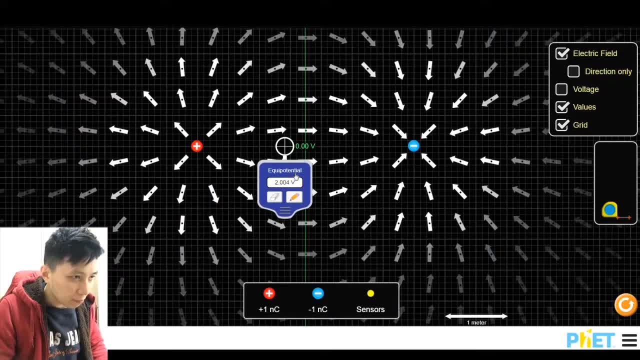 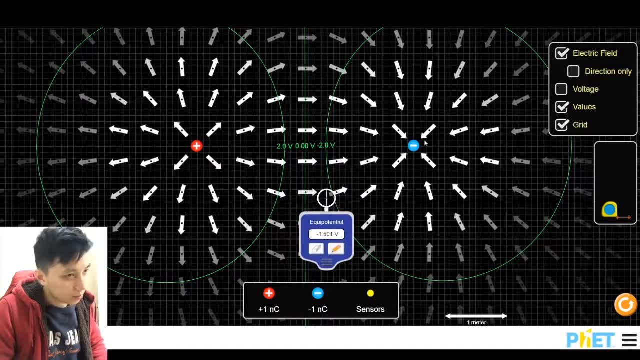 will be 0v. so, starting from this, i think that would be easy for us to work with and, as you know, if you get closer to the negative, it will become negative v obviously, and so you can see negative 2, positive 2v, and so that's. 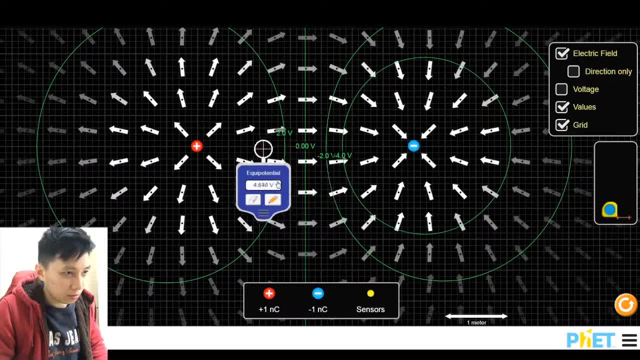 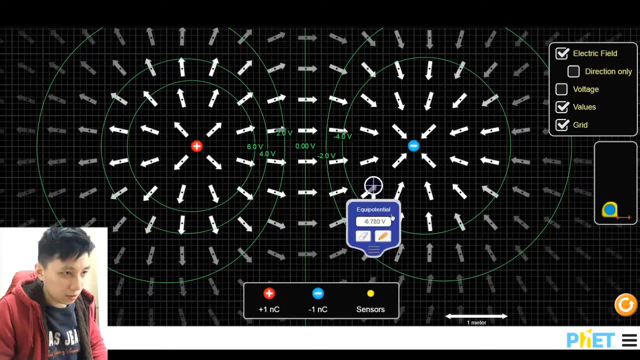 actually pretty much it you can. you should be able to guess the rest of them already, if any of us have just left out all these attached Upside Down. okay, 4 and then go for 6, and then here should be negative 6, negative 8. 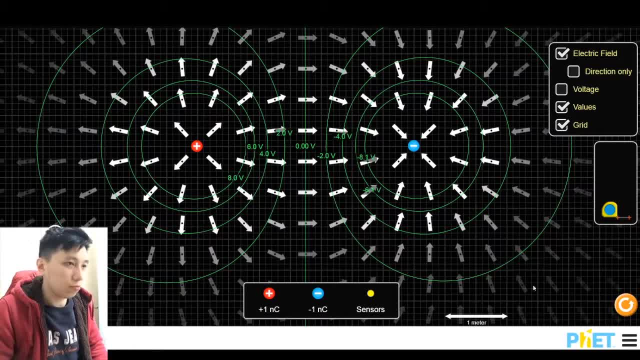 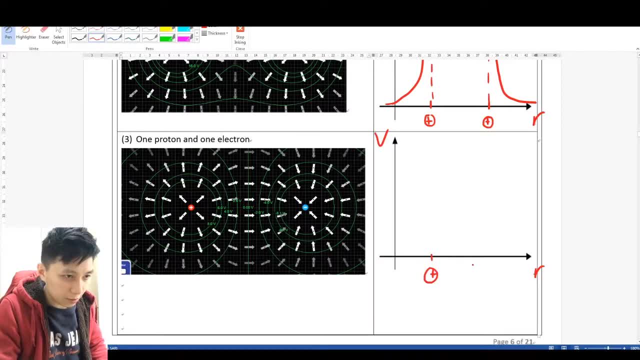 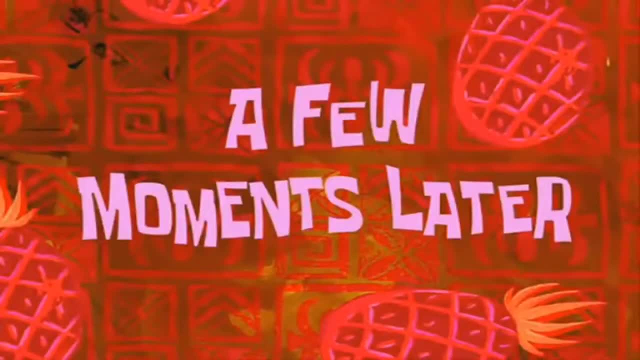 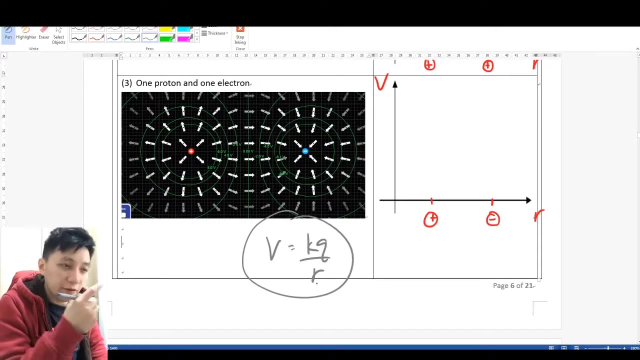 so anyway. so this is how the pattern would look like. and again, you should try to work on the graph now. if I say this is positive, this is a negative charge, how would they look like? try it yourself a few moments later again. because of this equation, no matter you are positive or negative, when out tends to 0, the V 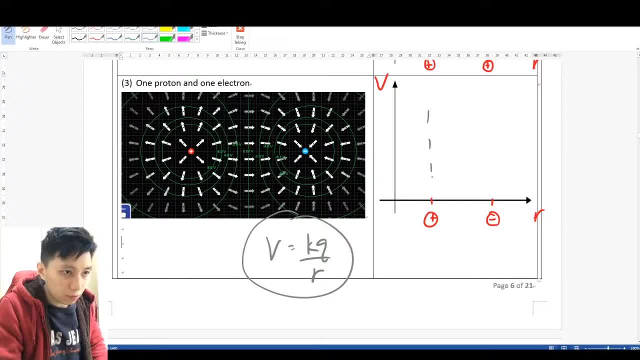 tends to infinity. so what we will do is again draw the up symptom, but this time because of the negative charge, we will have negative V, as you could expect, and so near the positive charge. I think you should know. look something like this positive value region and convert to 0 and then here for 100%, sure that you? 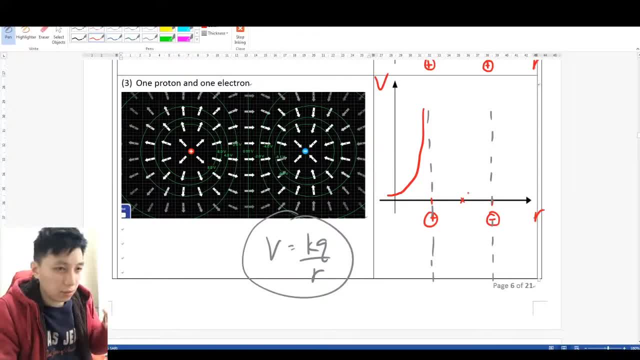 should have an anchor point which to remind you that you must pass through zero, and so this is something that it should look like okay, like a reflection, okay, and on near the negative charge, you would converge to the absent home, and that means you are going to negative infinity, and then you come back from. 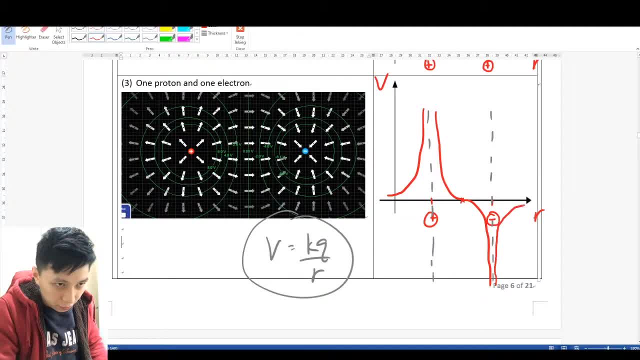 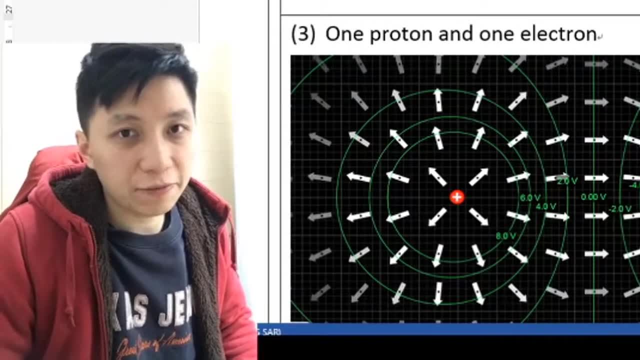 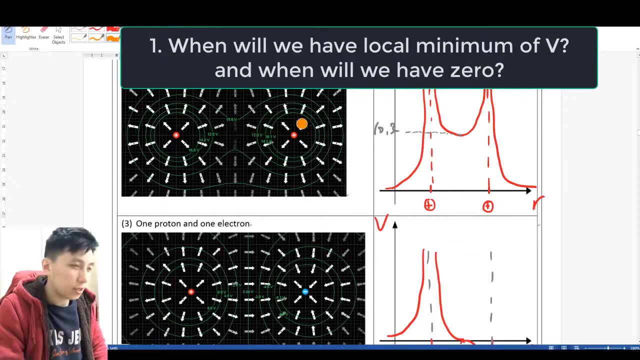 negative infinity again and converge to zero. okay, so this is how the pattern should look like. that's about it for the simulation activity. however, there are still a few more things you should pay attention, and let me remind you on that. so first again, when you have two proton, then you will never hit zero, right you? 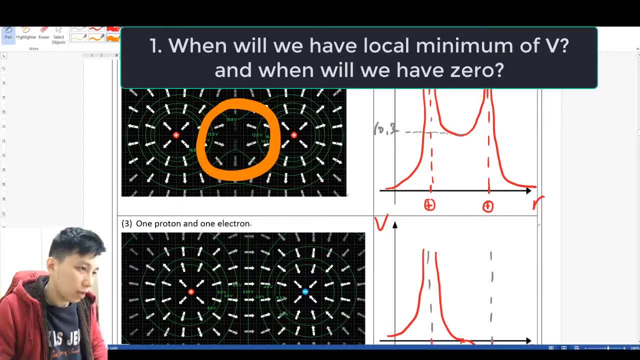 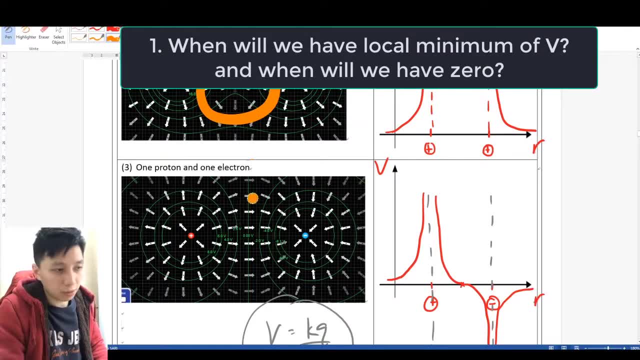 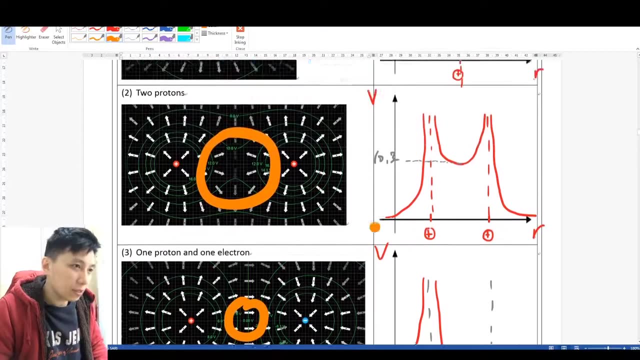 only would hit a local minimum here, and only if you have one proton and one electron, because one is positive and one is negative. so there is a chance where their potential in the middle somewhere, depending on their charge obviously, would become zero. so that's the first thing. second thing is, if you try to pay attention to the electric field line and 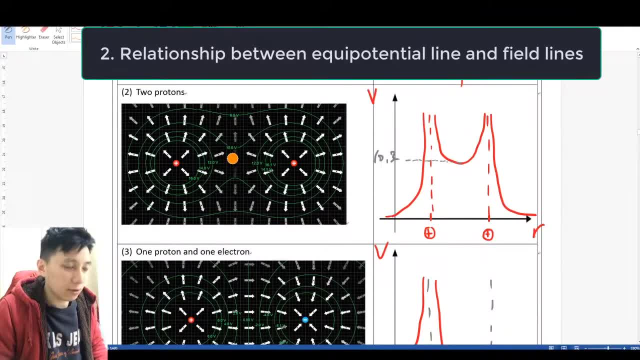 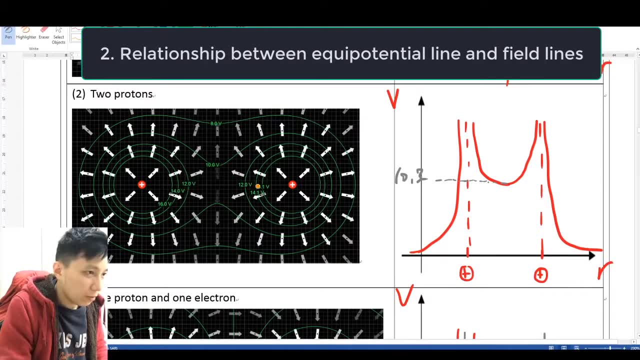 the equal potential line, they will have a relationship, which is true in general, that it is perpendicular to each other. so, for example, for case number two, you should be able to draw the electric field line like this maybe, and then like this maybe. okay, so you can see for the electric 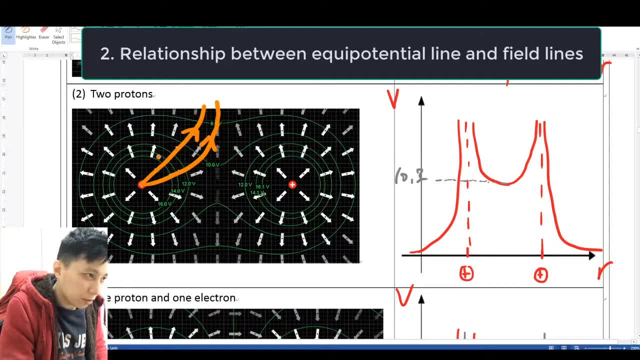 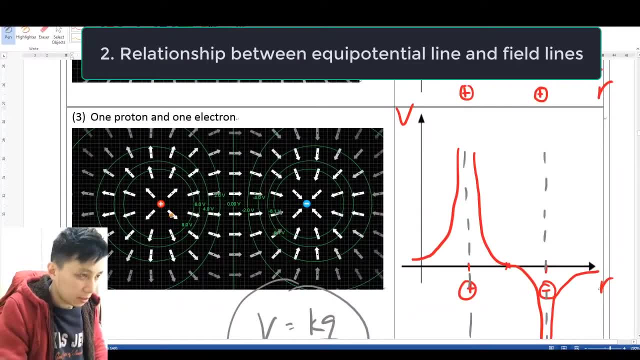 field line which is outward from the positive. it's always 90 degree to the equal potential line, same as maybe there's another case like one proton, one electron. then you should have electric field from positive to negative directly. so again you can see 90 degrees or 90 degree to the equal potential line and you can also draw. 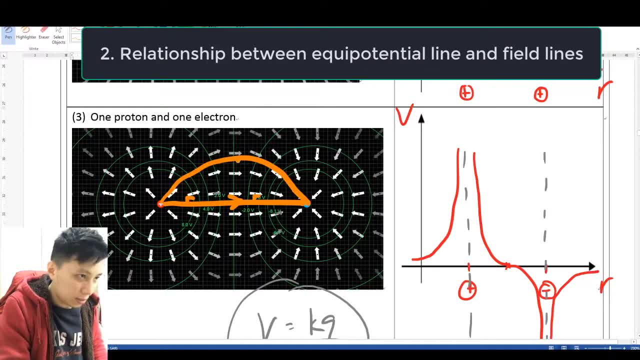 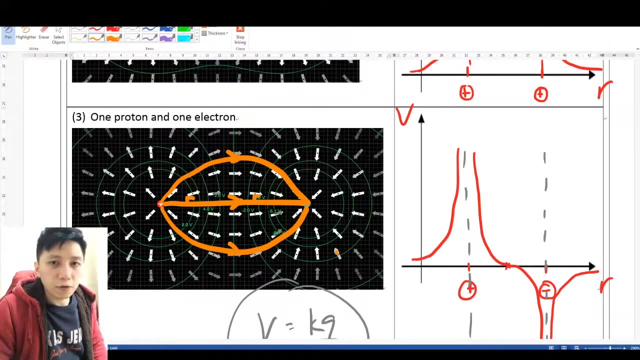 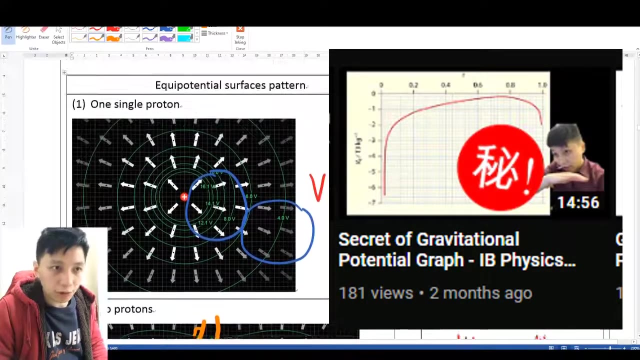 another one like this and these supposed to be 90 degree also. all right, similar at the bottom. so this is something that you you can visualize here and hopefully you can apply later on. lastly, if you recall, there's a trick that I taught you on gravitation, about the V against our graph potential line, and it's going to be a 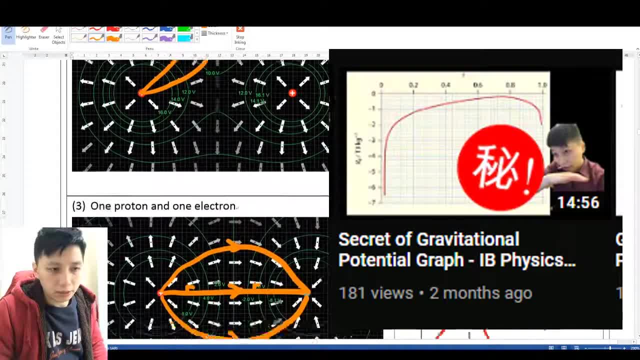 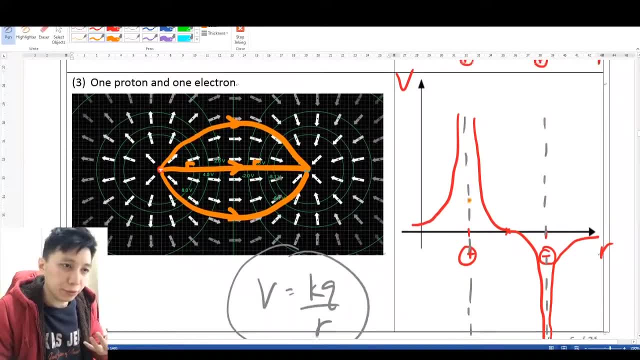 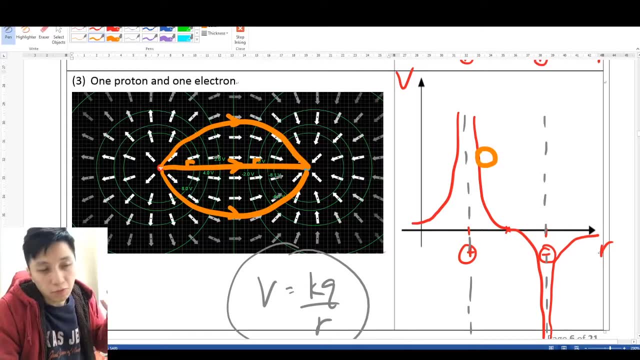 against the distance, and that is to think about the line itself on the graph is like the mountain, and so what you- what I asked you to do, to think about, is imagine there's a ball and on the graph that will happen to it is will be like: 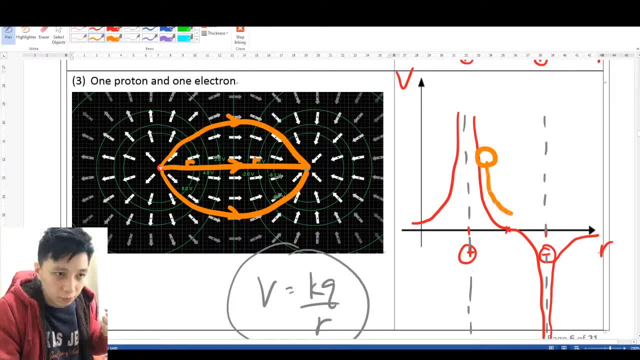 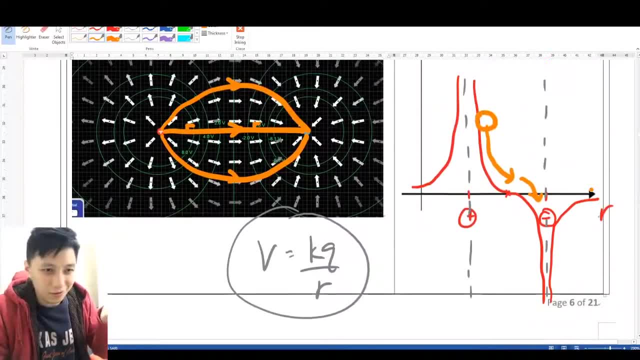 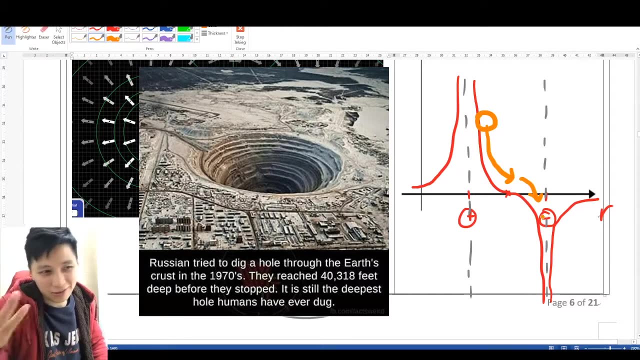 the ball on the mountain. so if you have a ball here, then it will roll down to the right and keep rolling. to this you know infinite hole or an infinite depth hole, and it can never come back. and same idea as in if you have a ball here in. 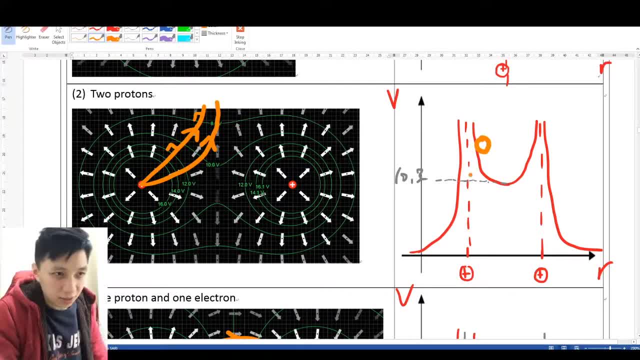 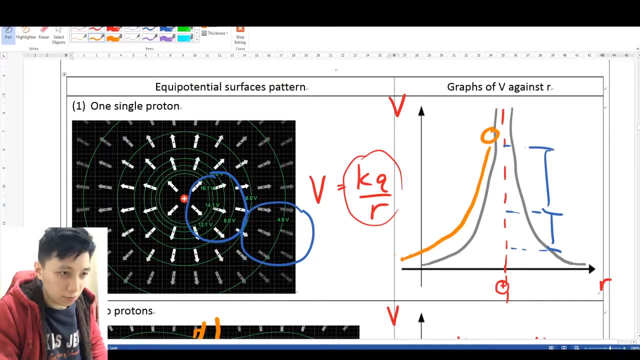 this pattern of mountain, then what it happened is it will go back and forth like this, probably okay, back and forth, and eventually, if you there's energy loss in a certain way, then it could rest at the middle right, which is the local minimum energy level. as for this, then it will just go to infinity. however, one important